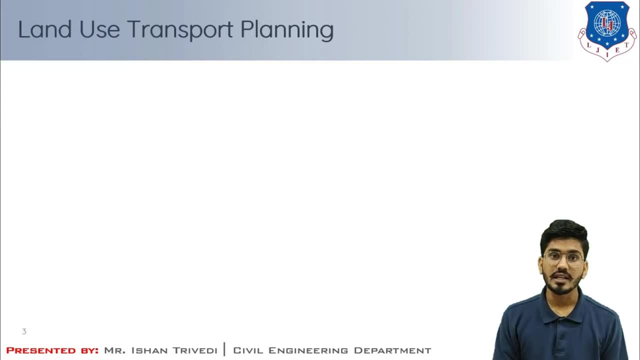 use options and recommends us the best pattern of staging various development. Here we need to understand the major components of long term strategic land use, transportation planning, where the urban development problem, their objectives, policies, all together with the forecast, or you can say the future prediction of population and environment. So we need 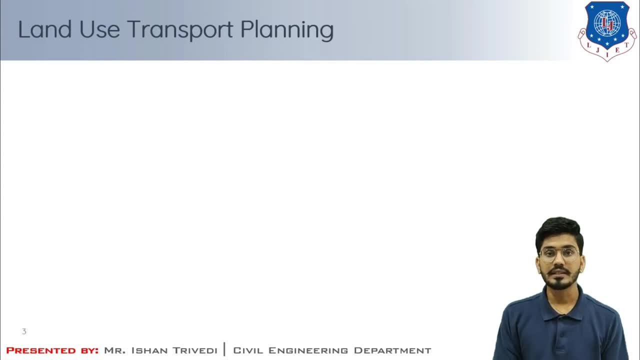 to understand the major components of long term strategic land use transportation planning, where the urban development problem, their objectives, policies, all together with the forecast, or you can say the future prediction of population and environment. So we need to understand the major components of long term strategic land use transportation planning. 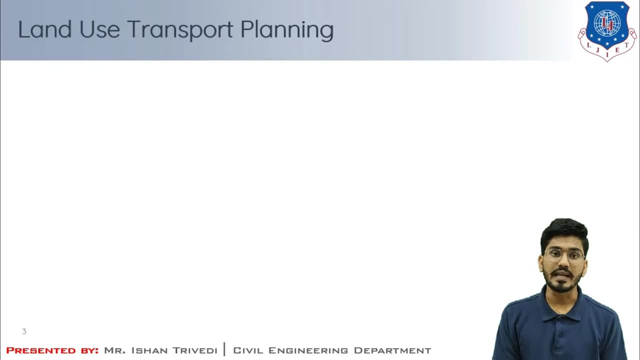 where the urban development problem, their objectives policies, all together with the forecast, or you can say the future prediction of population and environment. This means the purpose of portfolio planning, where the listing of bidings is based on central provision and its type. We have long term strategic land use transportation planning where you have access. 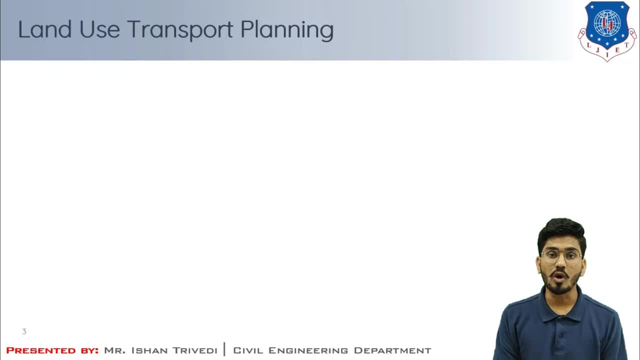 to planning and those are the main, those which we are going to discuss today. which 관련 is public location planning, with reports, objections and claims. So let keep going and we will realise the właściwie basis of local migration planning and why they are included in land use transportation planning, which 먹어� to take different. 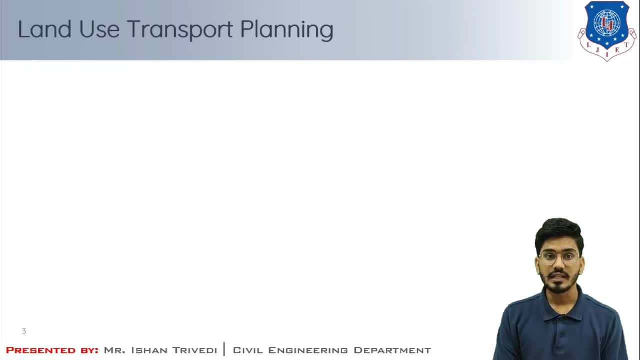 plan of land use performance, KPU, one is to have a linear calculation. скорее these land use activities are of socio-economic activities. After that, activities corridor by corridor, basis analysis is assessed to determine the major traffic implications. Then alternative land use transport system is evaluated. 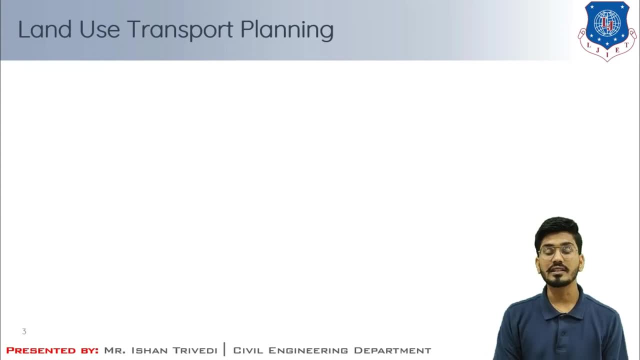 by the impact on the community and the environment. So this is what the land use transportation plan Now we will understand through a flow diagram. Here we have the land availability, geographical condition and environment constraint that we have. I have told you twice that is based on land availability. 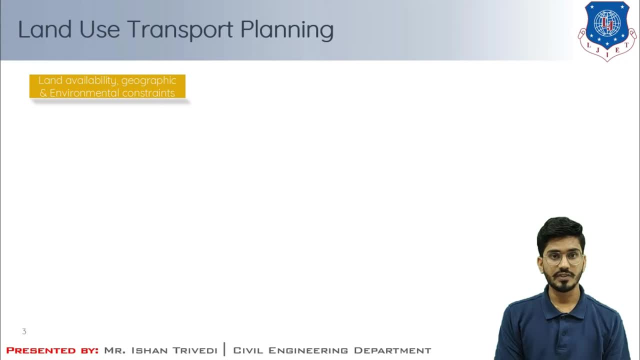 and the environment and the geographical condition, we have to form our activity. Then, based on that, we will form vision, goal and objectives that we want to achieve in the future. Now, here in this land. availability: there are two components, that is, of employment distribution and population distribution. 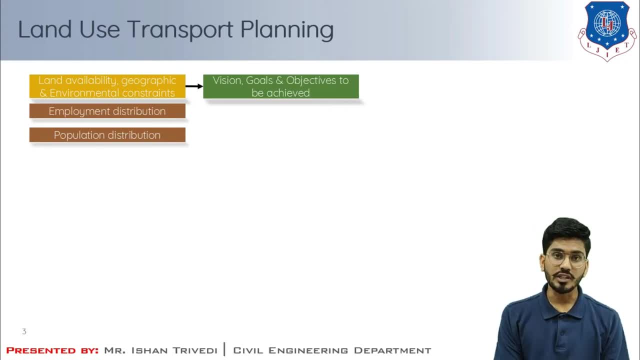 In any area, you will find the opportunity in urban area, In any urban area. there are two major concerns, and that is of population distribution and next is the employment distribution. Here this distribution requires a transport network, and of all these demands the plant is nothing but it is evolution of conceptual alternative plants. 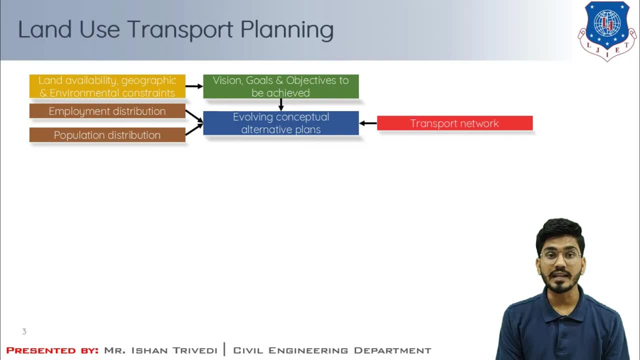 All these things require the alternative plants, which is suitable for the land availability and the environment constraint. Among of all these, there is one more need, that is, of data synthesis and distribution of land use based on the alternative plants. and there is another thing, that is transportation supply. 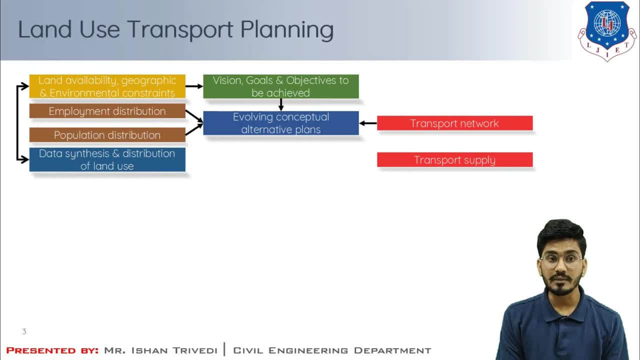 See, we have the population. We have the population, We have the economy, the aim to reach at the destination, that is of employment distribution. they need the transport network to commute from one place to another place and for that, what we need, we need a transportation supply. so, based on the conceptual plan, based on the land use availability, what we 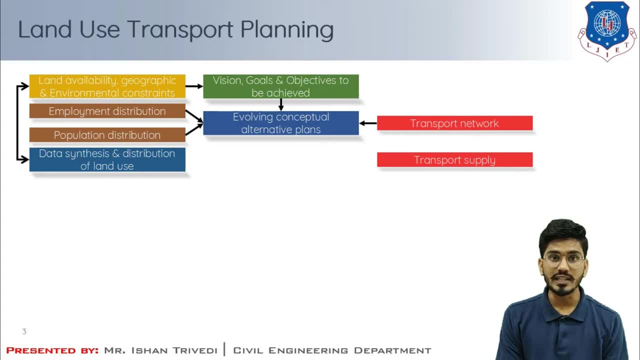 need. we need transportation supply and among of all these needs, what we need? i need to study travel demand models because ultimately, it captures the activity and the purposes that serves our activity. now these travel demand models are done, the data has been captured, then analytical and identification of major travel corridor is been identified. so, based on 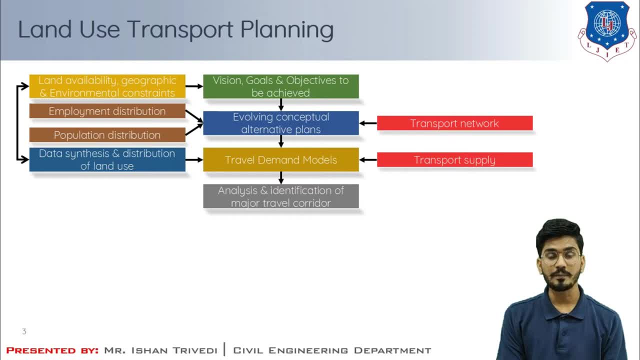 travel demand. what we get, we get the present situation, we'll forecast those things and what we'll get, you will get the major travel corridor and the futuristic demand here. these futuristic demand will lead to the urban transportation planning. again. these things are also implies to those land availability and environment constraint. furthermore, here i have options. that is the. 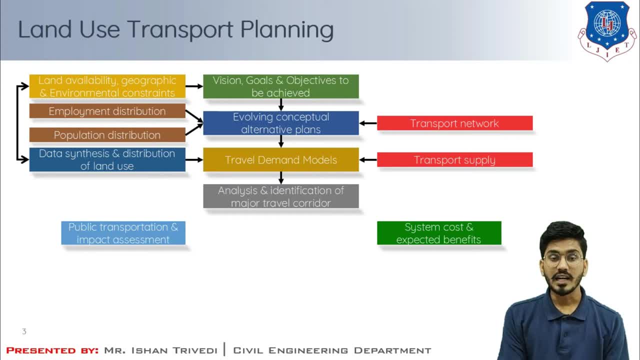 public transportation, impact assessment and the cost which are expected for those benefits here. among of all these three things, what i have to do i have to evaluate the alternatives and selection of base plan that we have evolving in the conceptual alternative plans. so once i have determined the 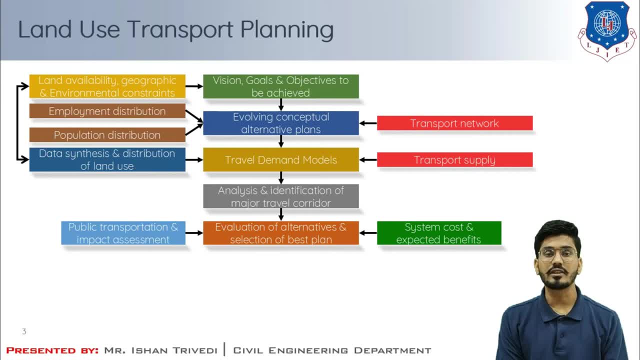 corridor. once i have assessed the public transport facilities, the fare structure, the cost involved in facilitating those public transport facilities, then what i need, i need based suitable plan to feed all these needs. now, from this plan i will get certain recommendation and strategies for the transportation system and at last i'll implement those plan based on the strategy and at last. 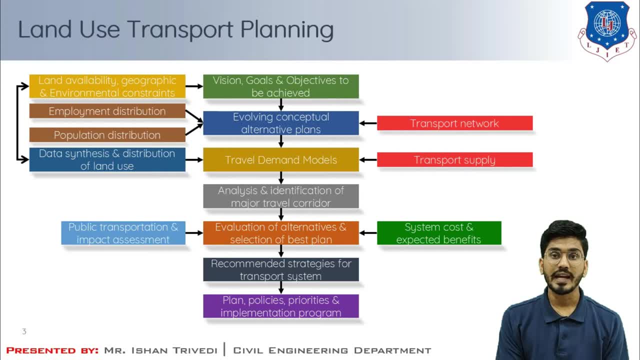 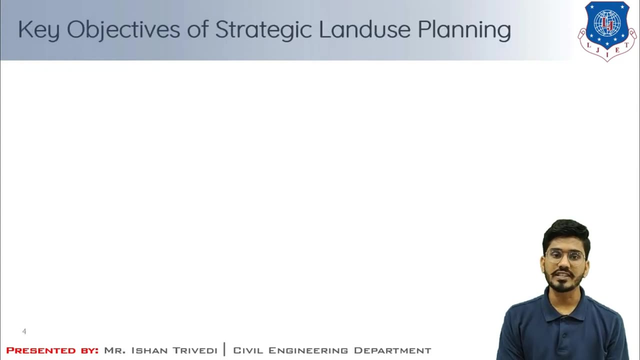 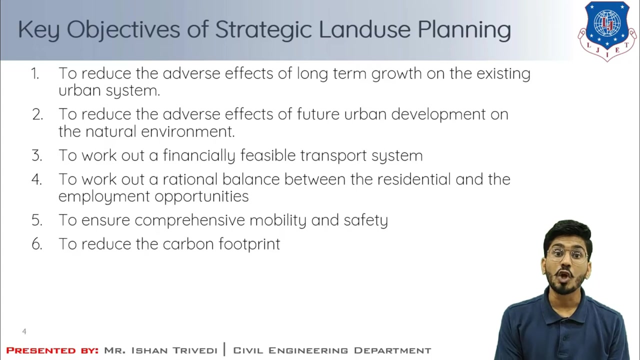 those plans, those policies and the priorities to establish this land use. transportation has been implemented by plan. so this is what the land use planning and its process now understand: the key objectives of strategic land use planning. here it is for reducing the adverse effect of long-term growth on the existing urban. 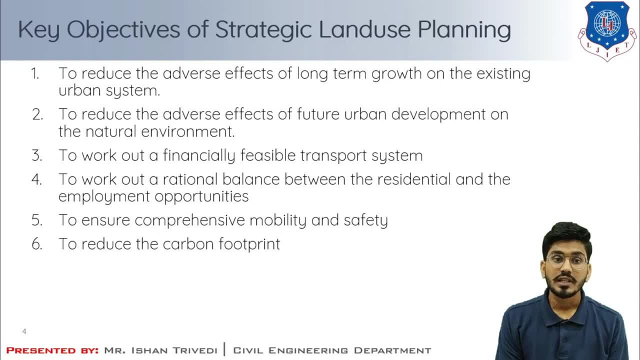 system, then it is to reduce the adverse effect of future urban development on the natural environment, then we need to work out financially feasible transport system. we cannot make transportation system in a sustainable way. we need to work out financially feasible transport system. we cannot make transportation system here and there, so we need to take care while spending this public money. 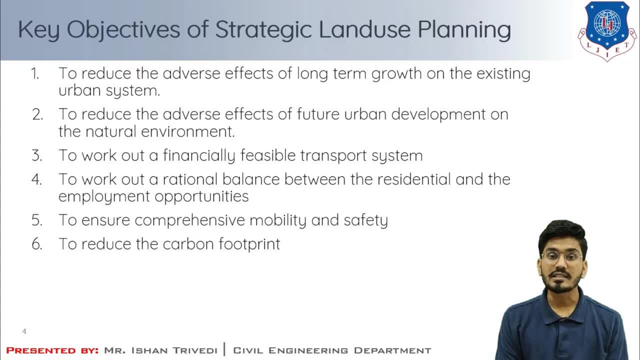 in the transportation system and it is compatible to environment with preference to the community. it is to work out a rational balance between the residential and employment opportunities so that the journey to work trip is contained. then to ensure the comprehensive mobility and the safety for all sections of people here, the poor class people, middle class or you can say working. 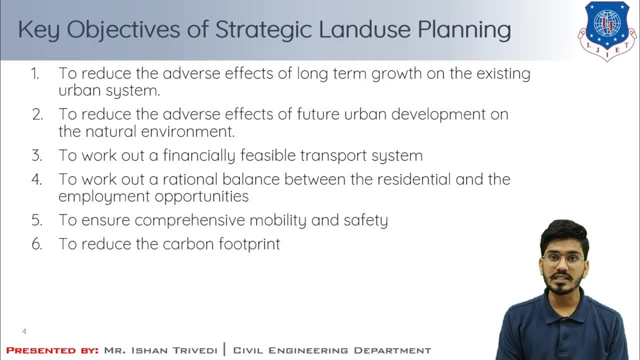 class people and the high class income group. all these category are classified and based on their needs. all things has to be provided, then, at last to reduce the carbon footprint by promoting the large share of public transport. here, what we need to take care, we need to just provide healthy living. 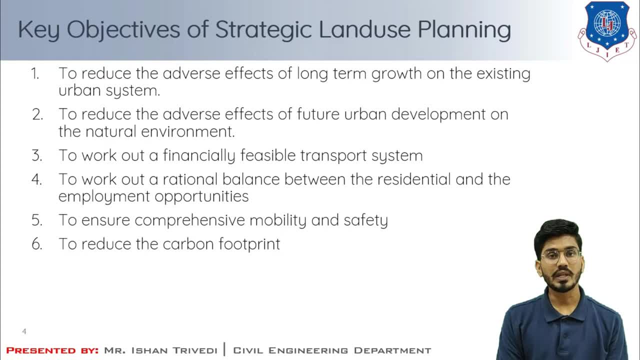 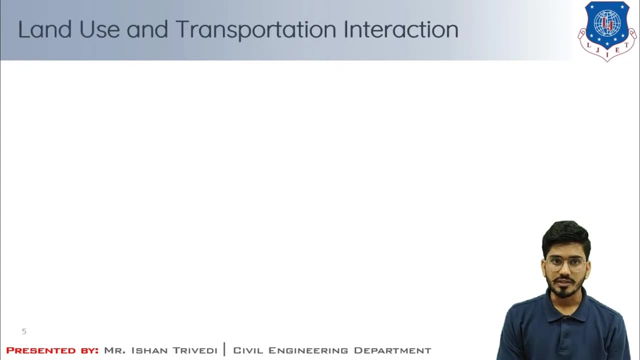 environment and we need to take care of the public transport and transport systems necessary for transportation in the society so that one can live easily. so this is what the land use transportation planning and their key strategies now based. on that we need to understand the land use transportation interaction here: the movement of people. 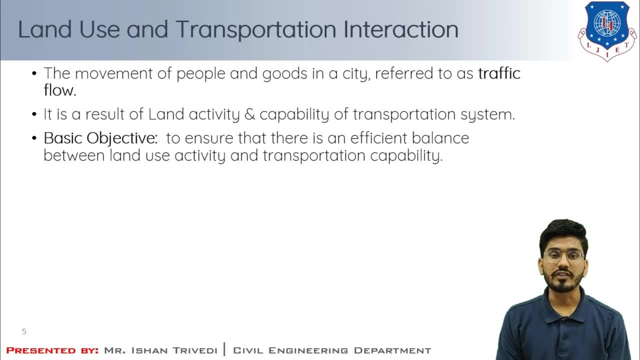 and the goods in a city referred as a traffic flow. it is the joint consequences of land use activity, what we call it as a demand, and the capability of transportation system to handle this traffic flow, which is called a supply. here the land activity is demand and the traffic flow is our supply, and there is 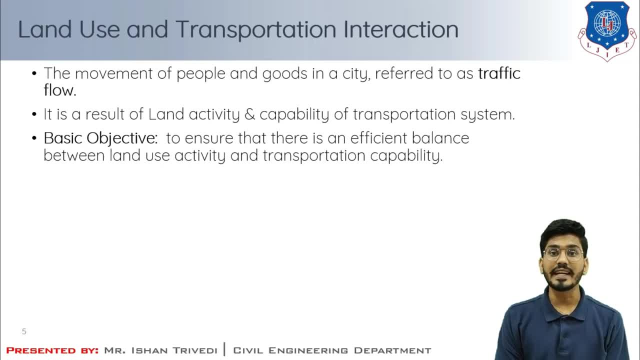 a direct interaction between the type and the intensity of land use and the supply of transportation facilities, which we are going to provide it here. one of the basic objective of the planning any land use and transportation system is to ensure that there is an efficient balance between land use activity and transportation capability. 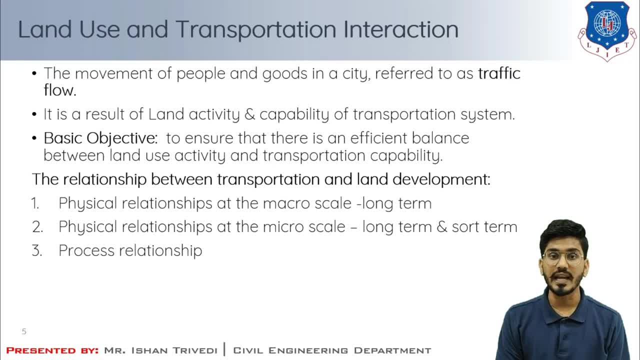 here there is a relationship between the transportation and land use development and we need to understand in this various context. first is the physical relationship between those components at macro scale- here these are of long-term significance- and the physical relationship between those components at macro scale- here these are of long-term significance. 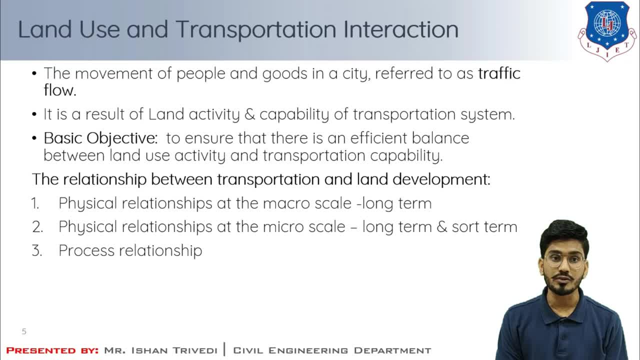 and generally consider as a part of planning process. again, it is a long-term goal and it has been done at macro scale- clear, and these are considered as a planning process tool. then there is a physical relationship at micro scale, which are of both short-term and long-term planning here. this has been 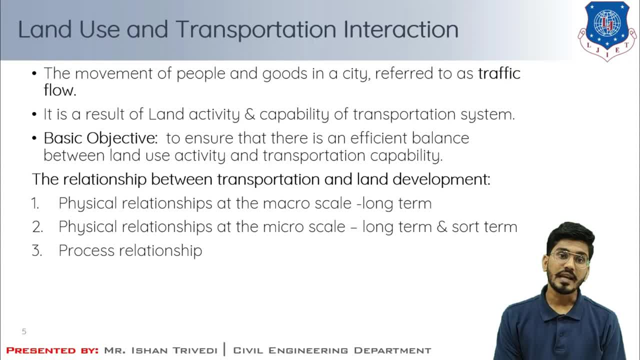 significant to highlight, or you can say, consider as a urban design, issues that we need to take care and, at last, the process relationship, which deals with the legal, administrative, financial and institutional aspect of coordinating the land use and transportation development. here, urban areas over the years have changed as a result of dramatic shift. 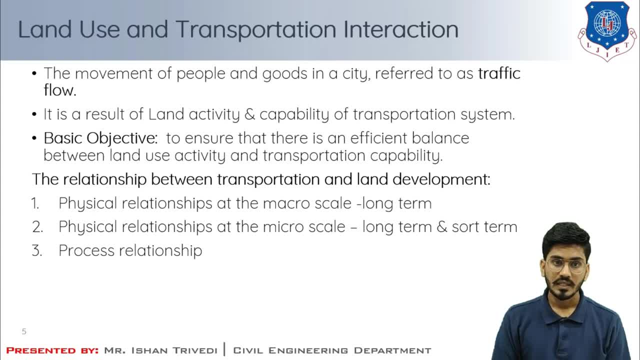 from the agriculture to urban development, they are now center of extensive financial influence and employment opportunities. their physical characteristics are changing rapidly as a result of new time and distance relationship which established by high speed travel and low-cost electronic communication. here the land use and transportation form a closed loop. 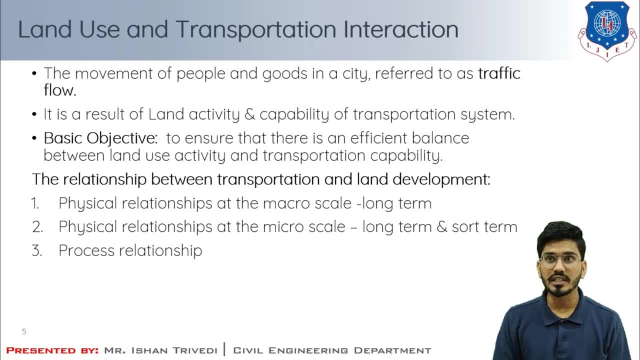 as I told you, which are the most other equilibrium system, which are the most most other equilibrium system, which are the most other equilibrium system, which lead towards land use and transportation configuration, which also stabilize here the land use potential is a measure of a scale of socio-economic activity, as I 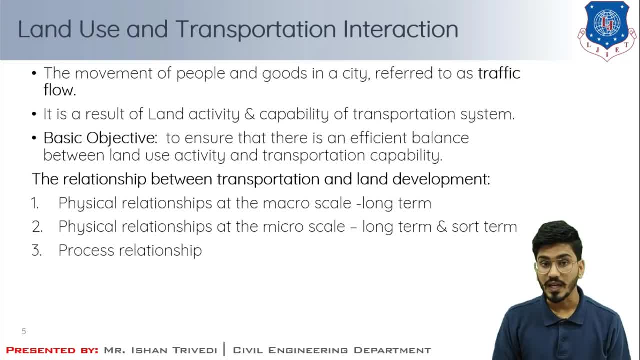 told you that take place on a given area of land. here a unique property of land use is its ability, or you can say a potential, to generate those traffic and hence it is appropriate to relate this land use potential of a parcel of a land having a particular activity to generate a. 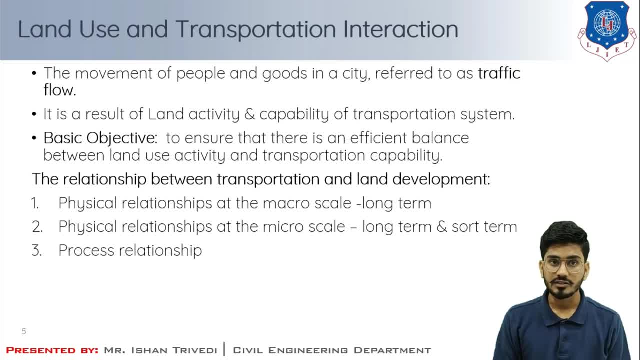 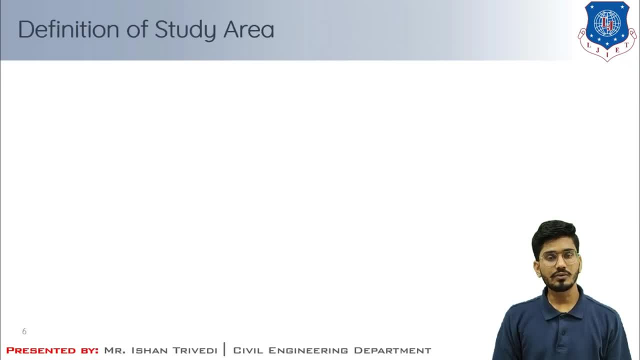 certain amount of traffic per day. this is what the land use and transportation interaction now, based on this theory, we need to study the study area, and for that I'll explain the definition of study area. in Urban Transportation Study, the study area should cover the anti-trench only the tariff and the trading area in Australia. 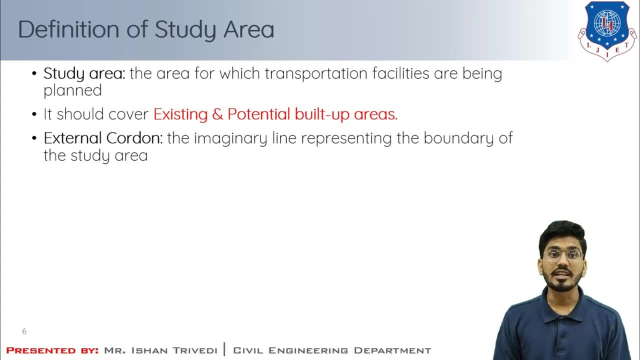 entire urban area containing the existing and the potential continuously built up area of the cities are which are likely to develop in the future. It is the area for which the transportation facilities are being planned. In Indian context, if I am telling you, this generally covers the area delineated as a. 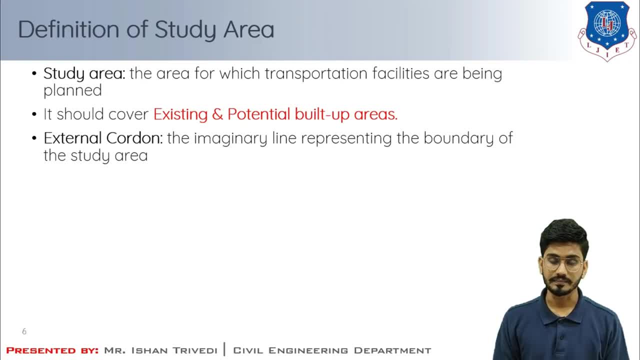 metropolitan area for planning and development, For example, Chennai metropolitan area, Mumbai metropolitan area, Ahmedabad municipal corporation area, Ahmedabad urban development area. So this can be the development which are in future. the planning is being done Here. one definition is there, that is an imaginary line which, representing the boundary of study. 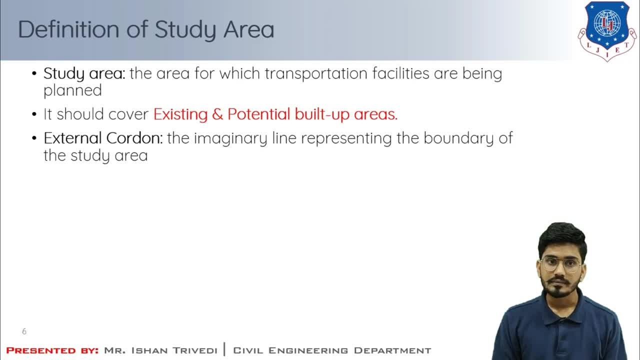 area is termed as external cordon line. Here again, I am repeating: It is a imaginary line. It is a line which is totally imaginary, which determines my study area. that is called external cordon line. It can be smaller, it can be of broader scale, it can be ward wise, zonal wise, or it can be. 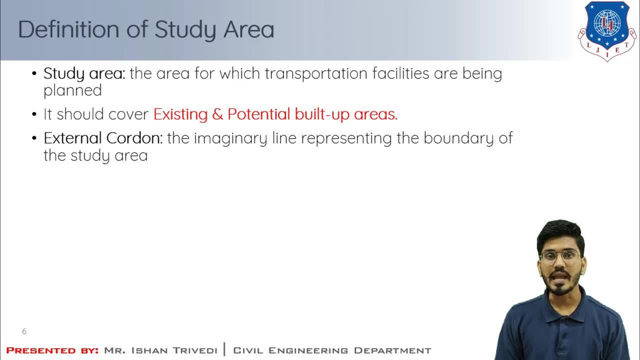 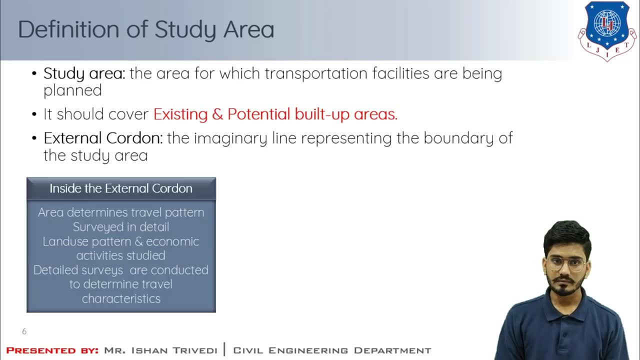 city level, AMC, ODA boundaries- This can be anything. So it is an imaginary line which defines my study area Here. there are two types of study area: one is inside the external cordon line and one is outside the cordon line. 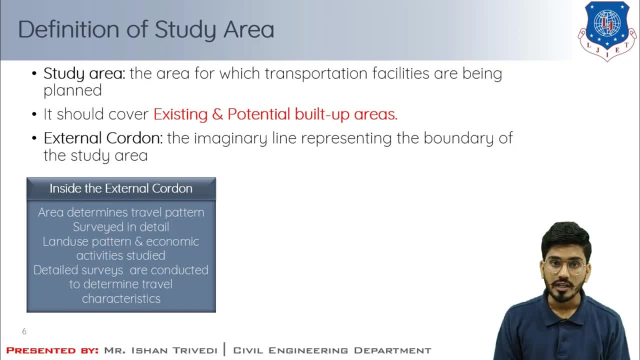 Now. first we will understand the inside, the external cordon line Here the area inside the external cordon line determines the travel pattern to a large extent and as such is surveyed in detail. Here the survey is done in detail. The land use pattern and the economic activities are studied here and detailed survey like home. 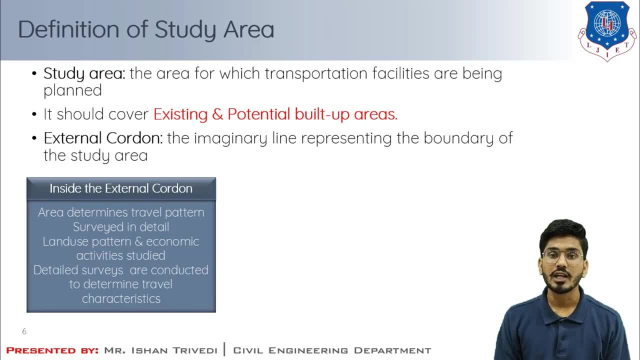 interview survey are studied here. Here the travel patterns are conducted in this area to determine the travel characteristics. Then there is another that is outside the external cordon line or outside the external cordon area, which is studied to a lesser degree in detail. Here the travel pattern from end to means, from origin to destination, the area outside, are 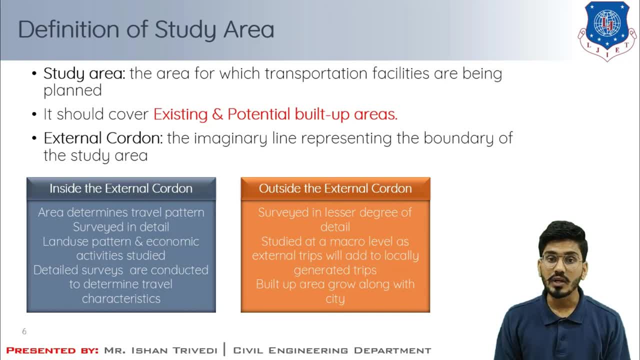 studied at macro level as the external cordon line. Ok, So these are the three types: external trips, which will add to the locally generated trips. The study area covered should be such that there are built up and are likely to, or you can say, futuristic area, along with the city which forms the core area and the people living. 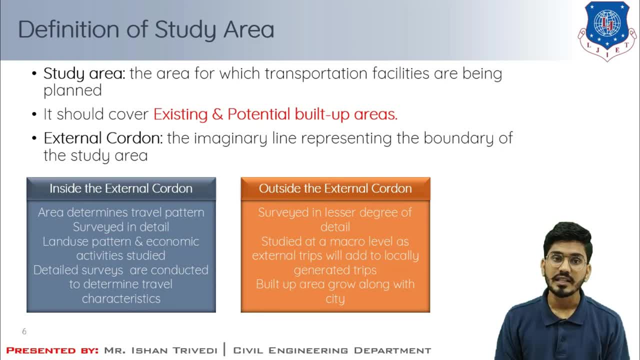 in within these areas have some dependency towards the city area and commute often in that direction. That means there will be developer of futuristic area and in that futuristic area there will be some core area and people will commute from the city area to those new area. 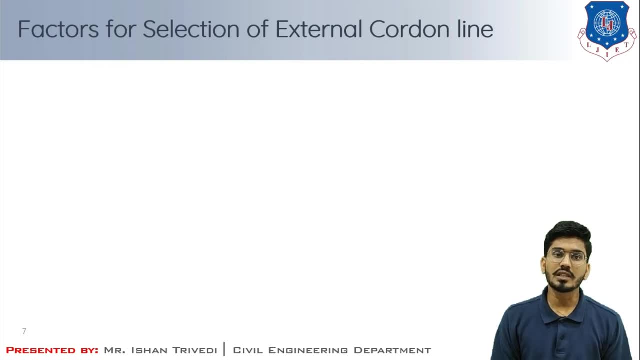 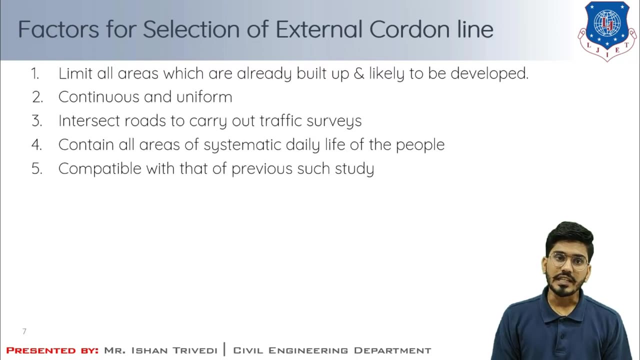 Now we need to understand the factors for the selection of the city external cordon line for the urban transportation study. First, is the external cordon line should be limit all the areas which are already built up and those areas which are considered or likely to be developed during the period.